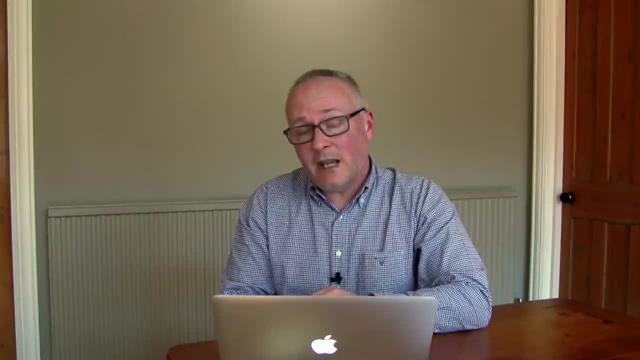 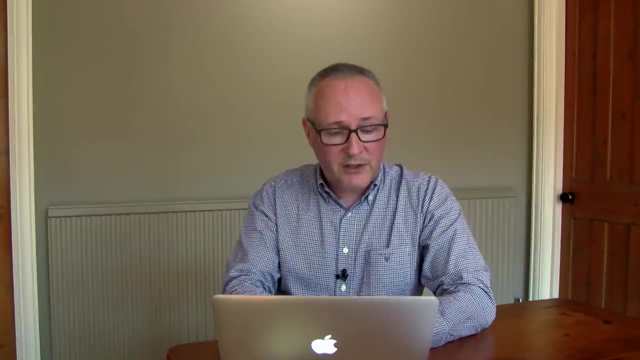 and, as usual, I'm going to be using Haskell, but you can basically do everything I'm going to show you today in any modern programming language that provides some support for the lambda calculus. So the example I'm going to start with is a simple increment function. 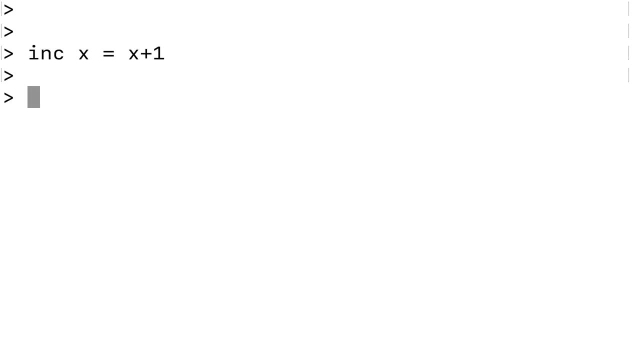 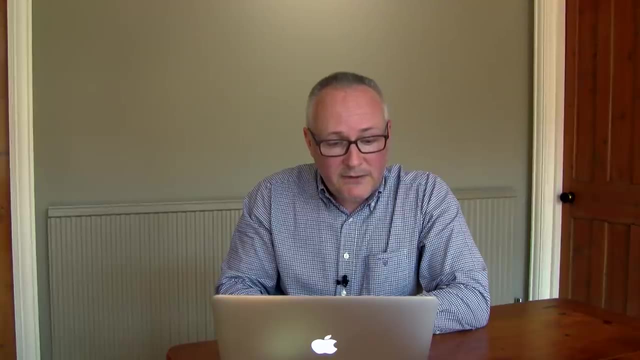 And we define it like this: increment of x is x plus 1.. So it just adds 1 to a number. So you can kind of have a look at the anatomy of this, so the structure of this, and we're doing three things: We're defining a name. 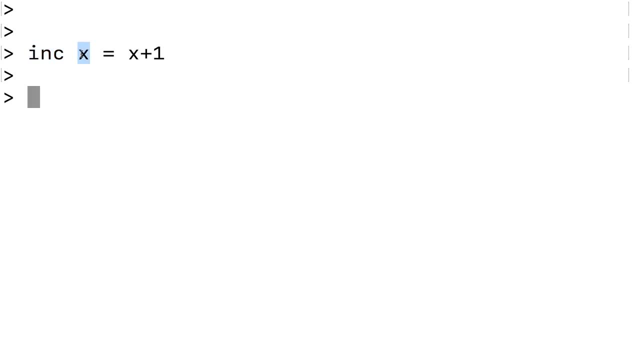 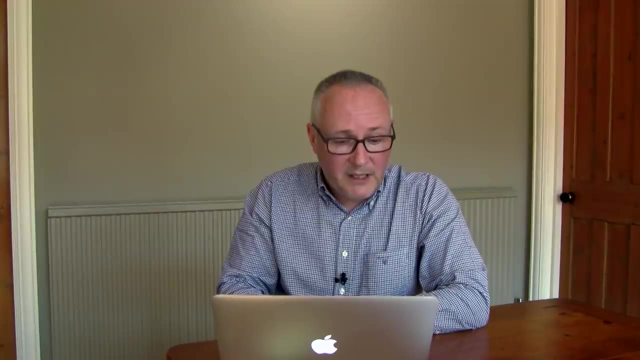 for the function. we're calling it inc for increment, we're defining a name for the input parameter x, and we're explaining how the output is calculated in terms of the input. So we can have a couple of examples of this: We could increment the number 1 and we get 2, or we 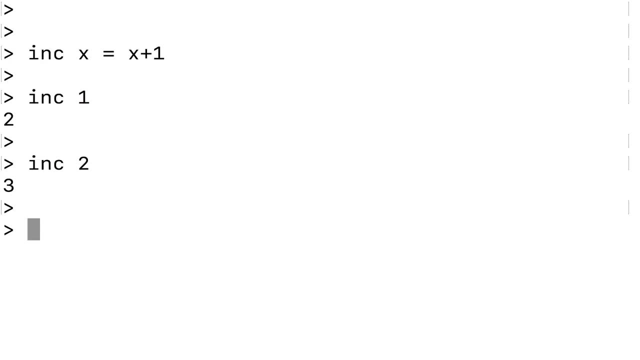 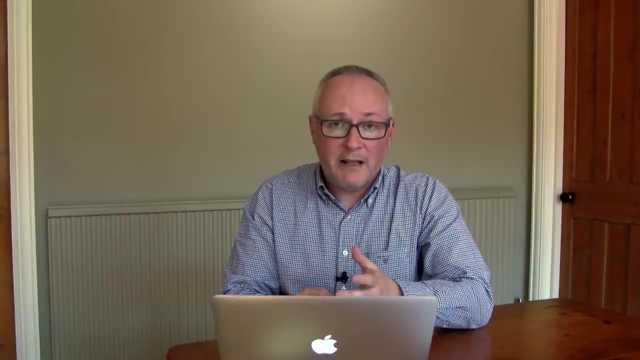 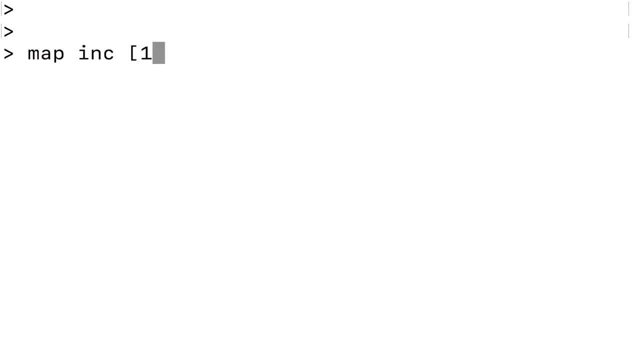 could increment the number 2 and get 3.. So it's all very simple and all very boring. So let's move on towards curried functions now, and the first step we want to take is the idea of applying a function to a function as an input. So let me give you a simple example of this. So what I'm going to? 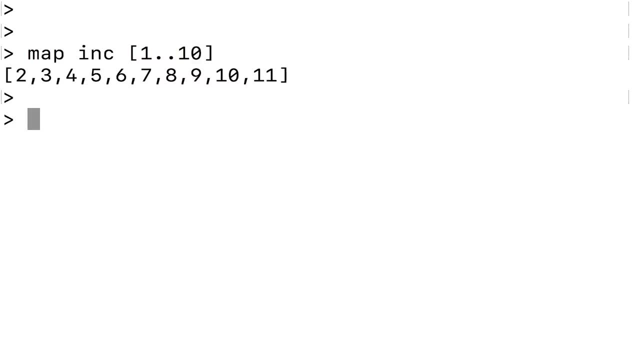 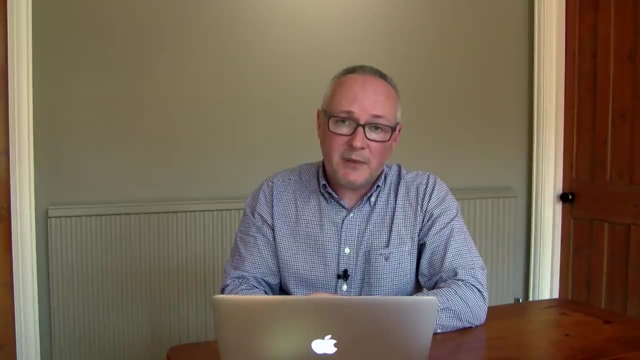 do is I'm going to map the increment function that we just defined over the list from 1 to 10.. So what map is is it's a function which takes two parameters. The first parameter is another function, in this case the little increment function that we just defined, and the second 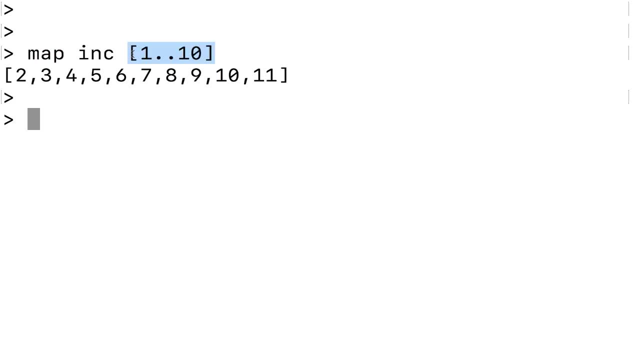 parameter is a list of things. So we're going to map the list of things and we're going to take the list of things- in this case a list of numbers from 1 to 10, and what map does is it takes the function here and applies it all the way across the list. So we're just simply 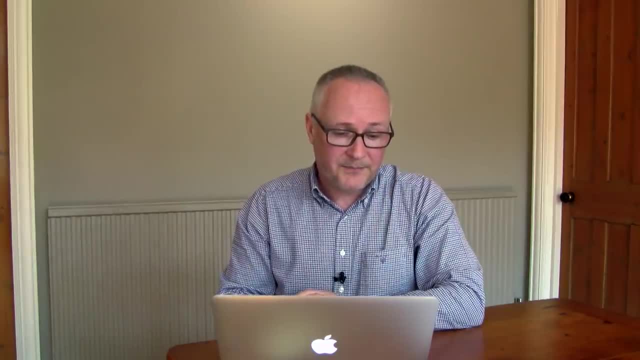 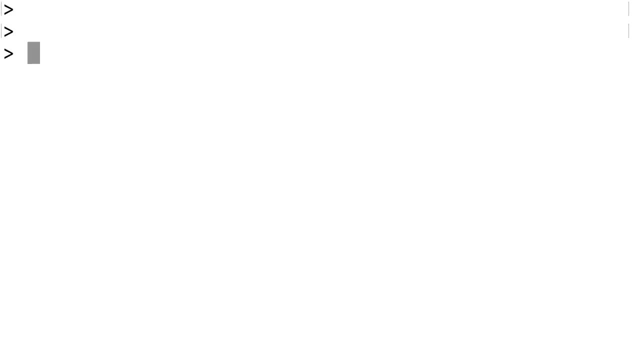 incrementing all the numbers from 1 to 10.. And map is called a higher order function because it takes a function as one of its inputs. So let's have another example of something a bit more interesting. Let's think about the idea of a function which has more than one input or more. 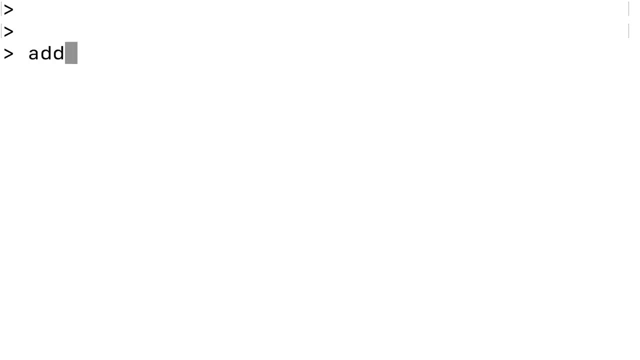 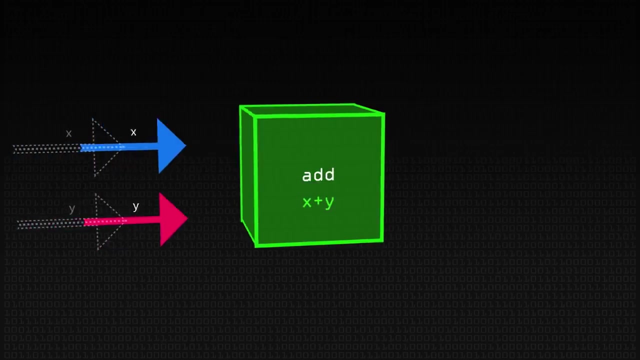 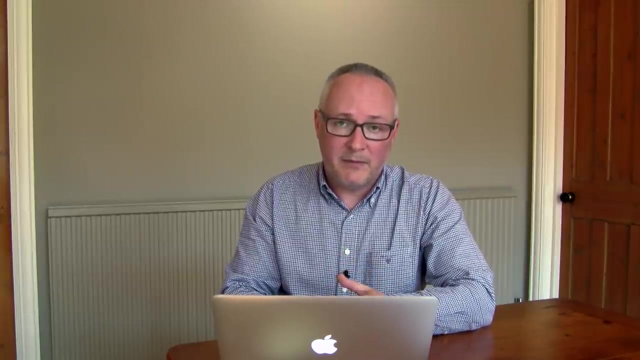 than one parameter. So we could define a little function called add, and we're going to take the two numbers x and y as inputs and then we're going to simply add them together, And the important point here is that we take the two numbers, x and y, packaged up together as a pair at the same time. 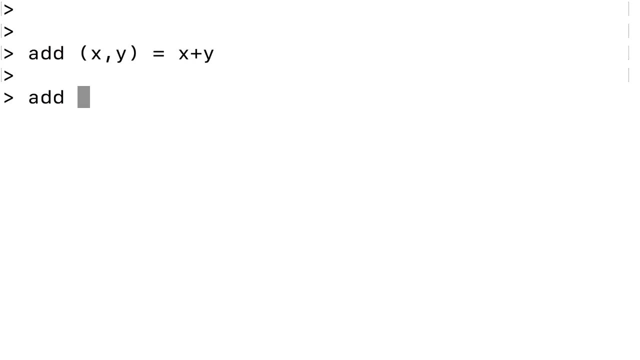 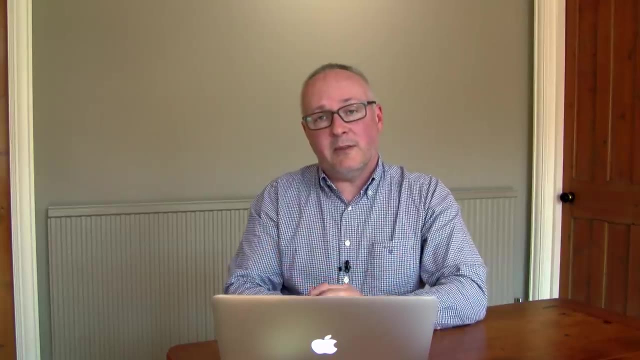 Okay. so what we're going to do then, for an example, is we could add 1 and 2 and give 3, or we could add 2 and 3 and give 5.. So all very simple and, again, all very boring as well. It's not really. 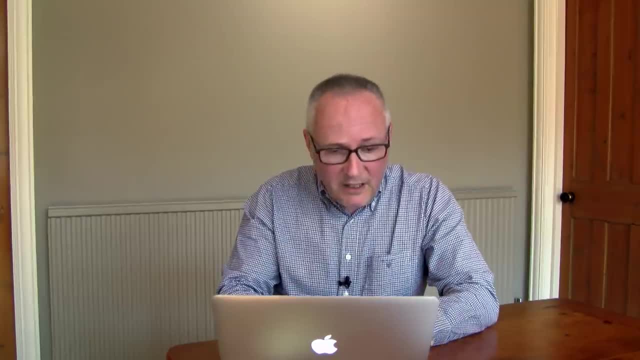 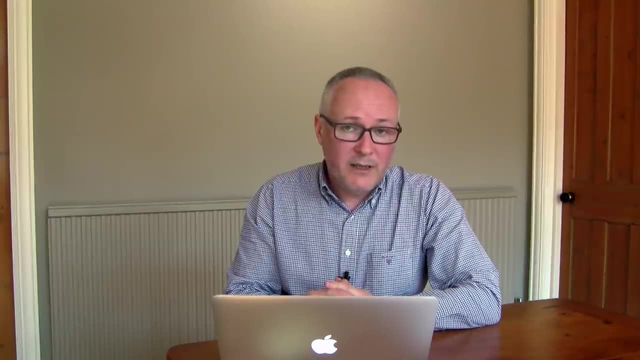 anything new at the moment. What, then, is a curried function? So a curried function is a function like add, which takes more than one input, but rather than taking them at the same time, packaged as a pair or a triple or something like. 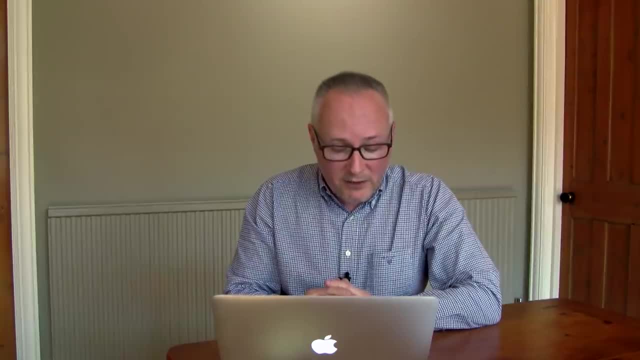 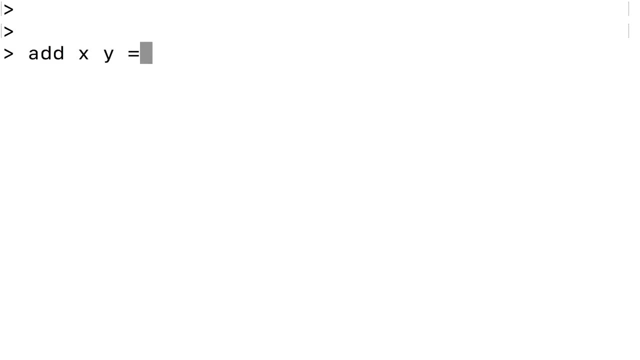 that it takes its inputs one at a time. So how could we redefine add as a curried function? What's very simple: we just take the brackets out. So rather than saying add of xy is x plus y in brackets, we just say add of x and then a space, and then a y is x plus y. 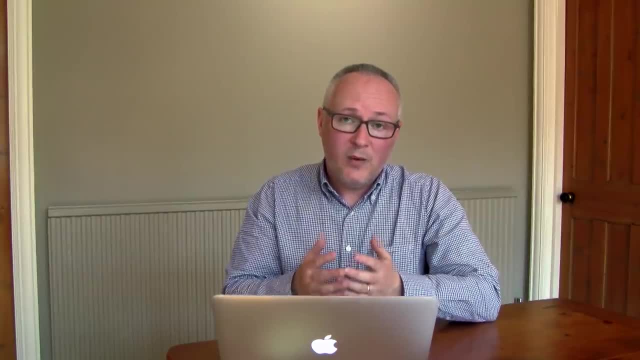 So what we're going to do is we're going to take the two inputs x and y, and we're going to take the two inputs x and y, and we're going to take the two inputs x and y one at a time. now. 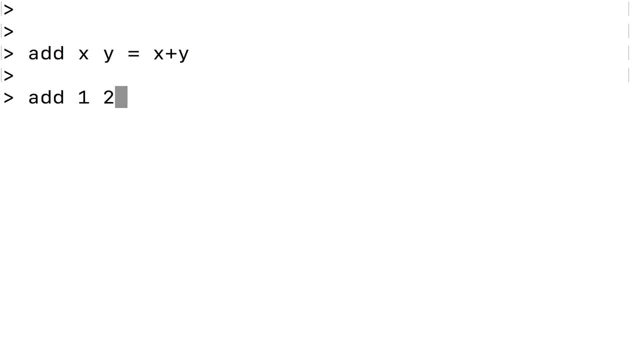 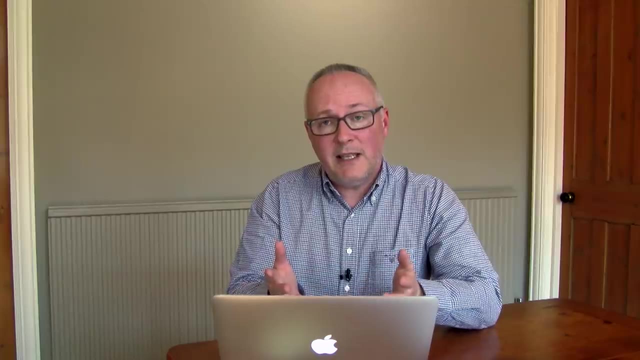 rather than at the same time in a pair. And then we can apply this function in exactly the same way as before, and we just give it two inputs, like 1 and 2, and we get 3.. Or we could say: what's 2 and 3,? 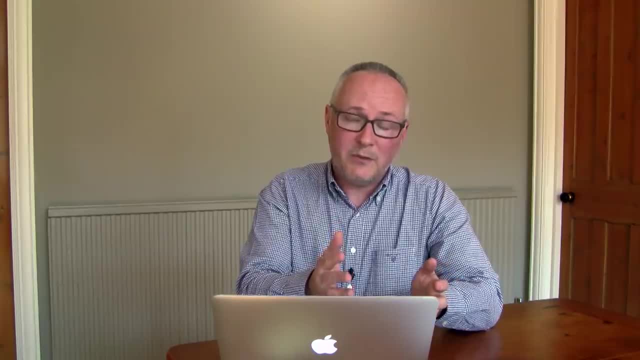 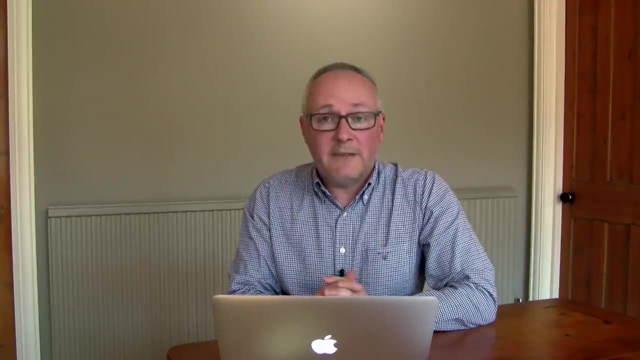 and we get 5.. Okay, so it looks basically exactly the same as the regular addition function, except, rather than taking a pair of inputs at the same time, it takes two inputs, one at a time. What's the point of defining functions in this curried manner? Well, the point is that you don't. 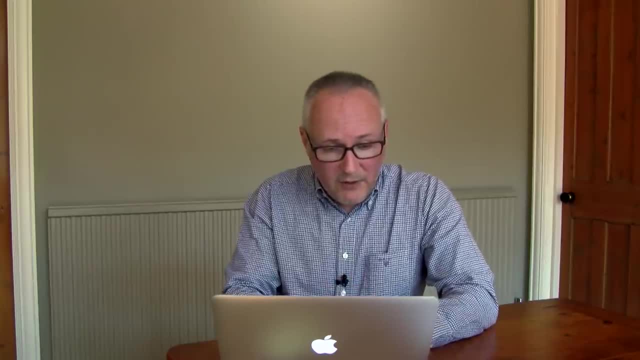 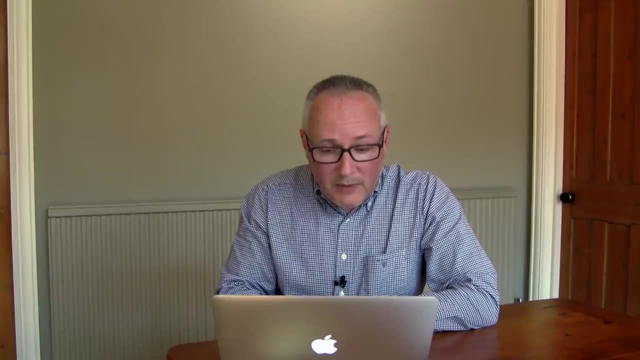 need to give them all of their inputs. So, for example, if we did add of 1, and we see what it says, oh, we actually get an error here. So why do we get an error? So we get an error because this: 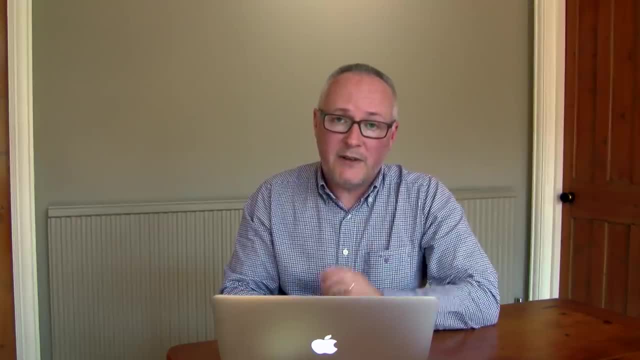 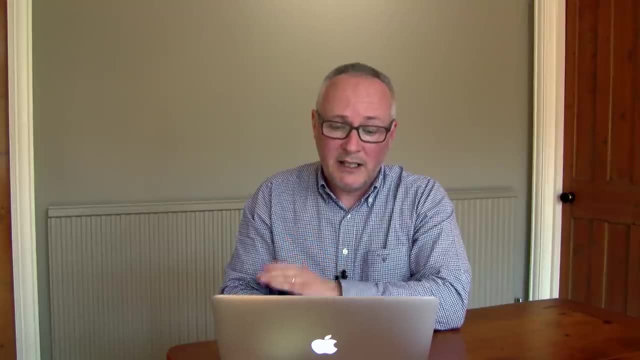 is still expecting its second parameter. So if I apply add to a single number 1, it doesn't know how to do the addition yet because we haven't given it a second number. And that's what it's saying here. It's trying to put in a number 1, but it doesn't know how to do the addition yet because we haven't given it a second number. And that's what it's saying here It's trying to. 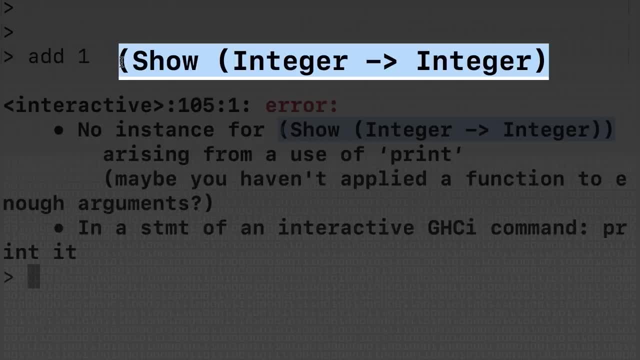 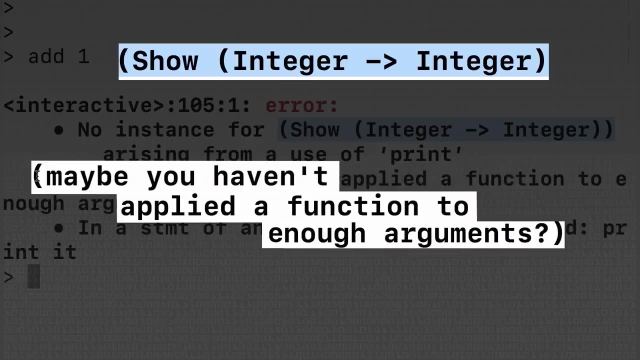 print a function here. So it says: I don't know how to show a function from integers to integers. Or, if you want a more slightly comprehensible message, it's saying: maybe you haven't applied a function to enough arguments. Okay, so with a curried function which takes its input, one at 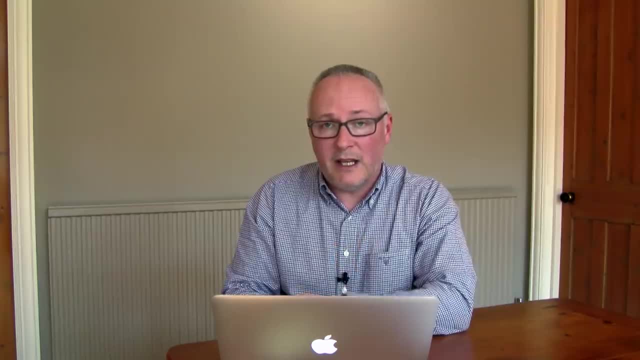 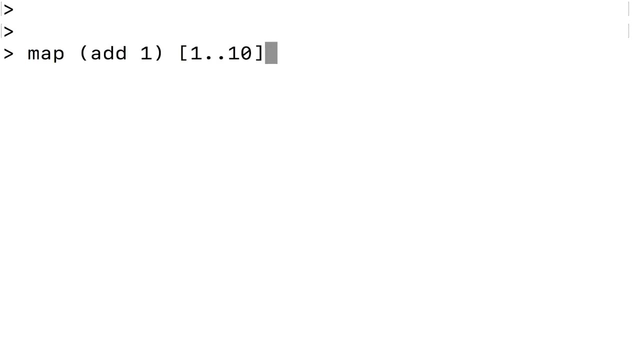 a time, you can partially apply it to a subset of the inputs. So what could you actually do with a function like add 1?? Well, we could map it, for example. So here is a way of incrementing a list of numbers. So what we can do is we can add a function to a function like add 1.. And we can. 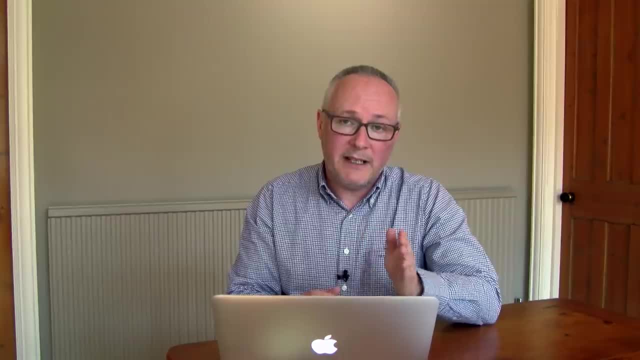 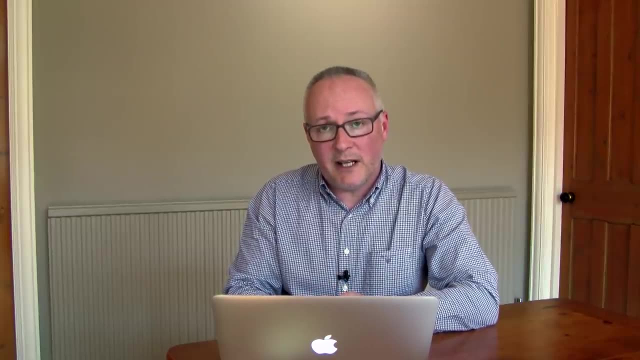 map the list of numbers without defining a custom increment function. So previously we defined inc of x as x plus 1, and then we mapped it. Here we're using the add function, which is curried because it takes its inputs one at a time And all we're doing is giving the add function. 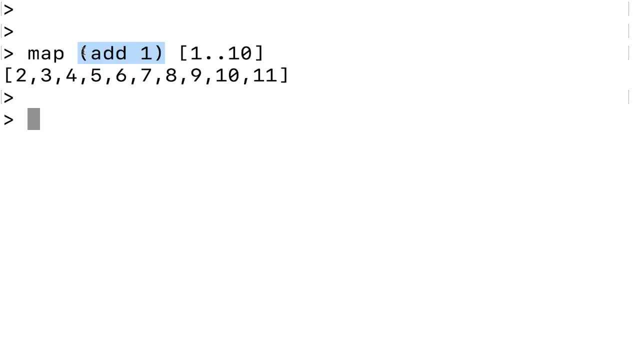 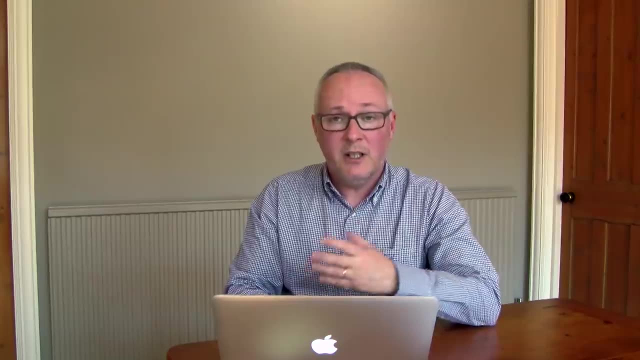 one parameter here, And then it's a function which expects its second parameter, And then it will map that all the way across the list. So we get the same behavior using this general purpose addition function without having to define a custom increment function. So you can ask yourself at: 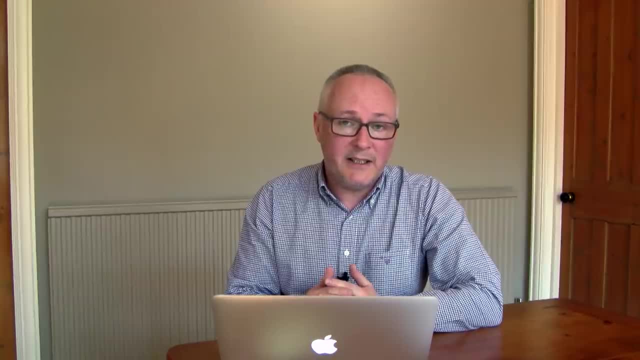 this point, what's adding a function to a subset of the inputs? Well, we can do that by actually going on with a curried function. When I say it takes its inputs one at a time, what does that actually mean? So let's kind of look at this definition again. So here's the 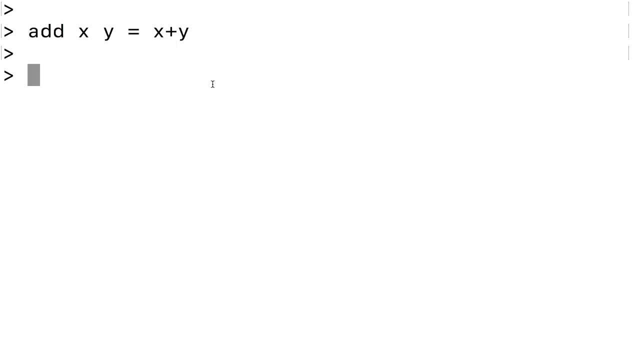 definition we had. Add of x- y is x plus y. What we can do is do a simple lambda calculus trick here: Rather than having the two inputs on the left-hand side of the equals, let's move them across the equal sign to the right-hand side of the definition, And we'll do this in two steps. 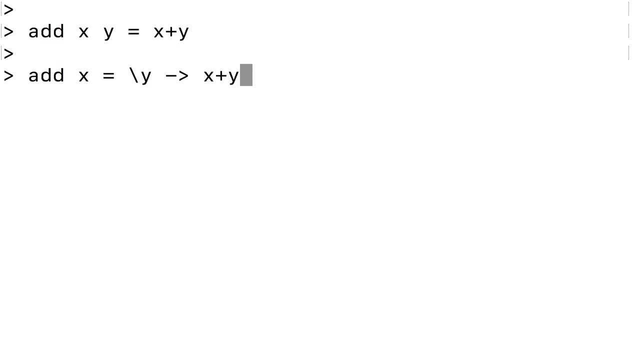 So what I'm going to do is I'm going to say: add of x is lambda, y arrow x plus y. So what I've done here is the y is no longer on the left-hand side of the definition here, Now it's on the right-hand side of the definition. So what this is saying is if 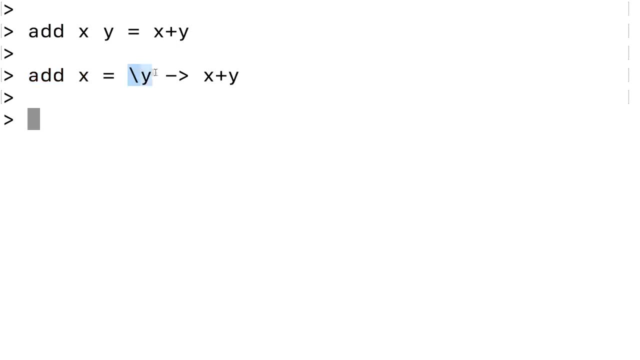 you add a number x, then what you get is a function which is waiting for a second input, y, and then it's going to give you back x plus y. And this expression on the right-hand side here is called a lambda expression. It's a nameless function And it's got the same kind of anatomy. 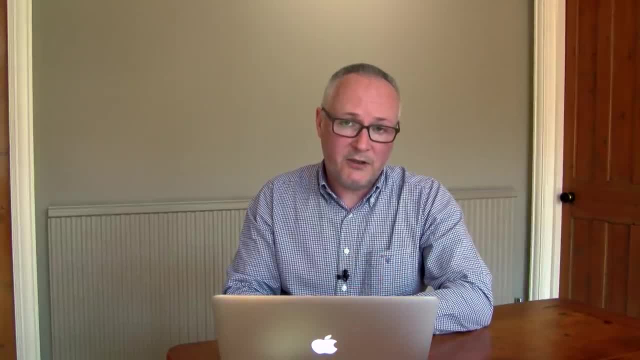 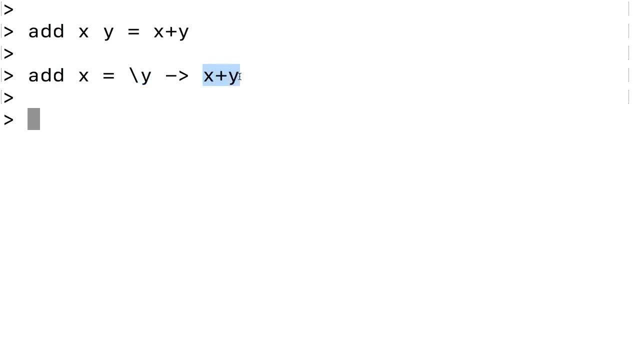 as a normal function definition, And it's going to give you back x plus y. And it's going to give you back x plus y, except for the fact that you don't give the function a name. So if you look at what's going on here, we're taking an input parameter called y and we're giving back the. 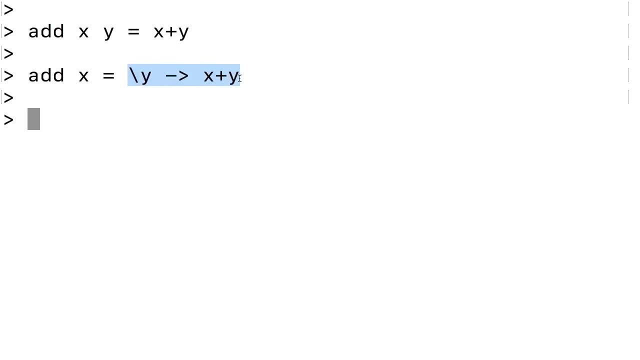 result: x plus y. But nowhere in the blue box here have we actually given the function a name. It's a nameless function, And then we can actually play the same game with the other input as well. So rather than having x on the left-hand side, we can move it across to the right-hand side. 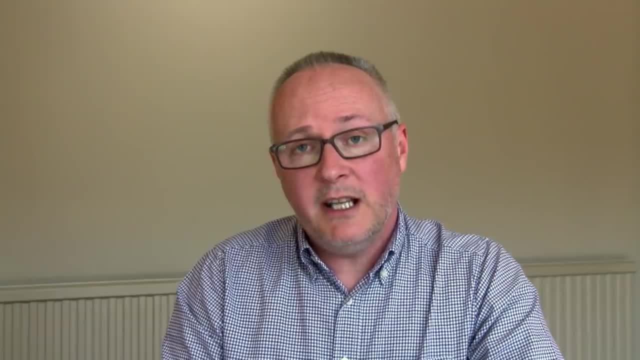 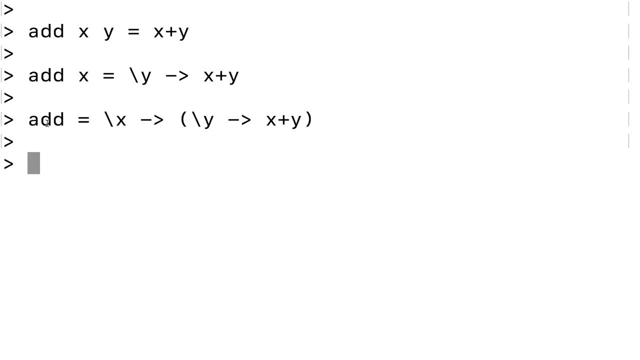 And here we have our definition of our add function in a more primitive way, And this is what we're trying to understand in a quite fundamental way. what's going on with Curried functions? What we're saying is that the addition function is defined to be the function which 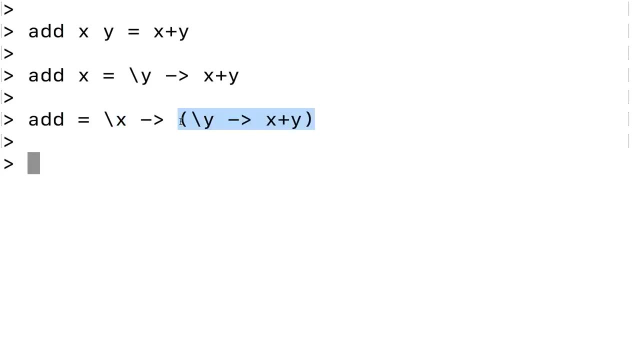 takes an input called x and what you get back is another function, And that function takes an input called y and then gives you back the result x plus y. You can ask yourself: where does this idea of Curring come from? Well, it's named after Haskell Currie, who was a mathematician and 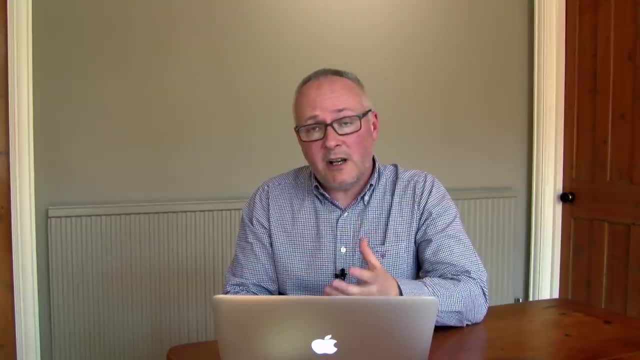 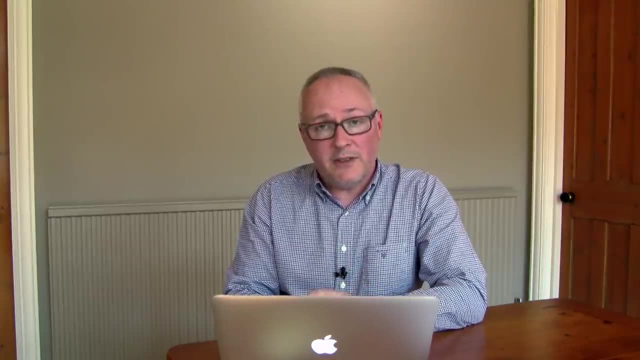 logician who studied these kind of things, But Haskell Currie himself. he worked on a lot of these kind of things And it wasn't the person who actually invented this notation or this idea. He attributes it to someone else called Moses Schoenfinkel, who was also a logician, and 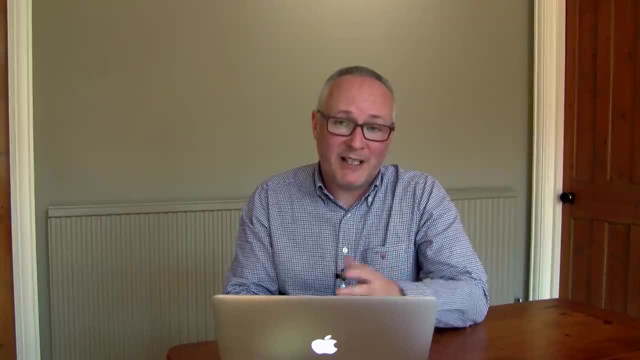 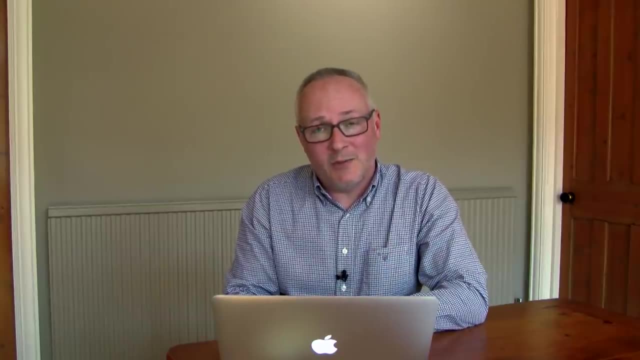 mathematician working around the same time. Schoenfinkeling is quite a hard word to say. I've had to practice it quite a lot even to be able to say it today. It's not a word which is very easy to say, Whereas Curring kind of just trips off the tongue. It's a nice easy word to say, So Currie. 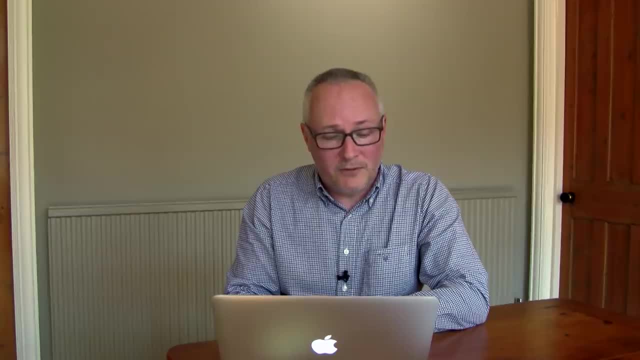 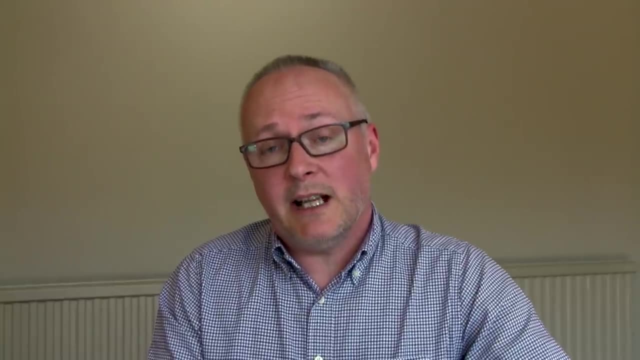 got the credit for it, But really probably Moses Schoenfinkel is the one who first studied this idea. So, just to wrap things up, I want to give you an example which shows you how to do this, And I'm going to show you a little bit of a video that shows that actually Curried functions are quite 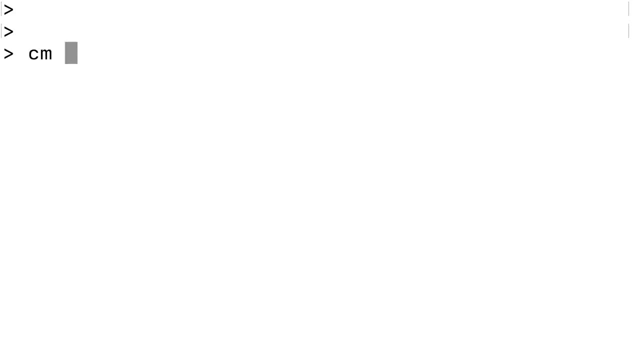 natural in the real world as well, not just in computer science. So we think about a cash machine. What does a cash machine do? Well, it takes three inputs, Typically. you put your card in, you put your pin number in and you put a request in, And then it's going to give you some. 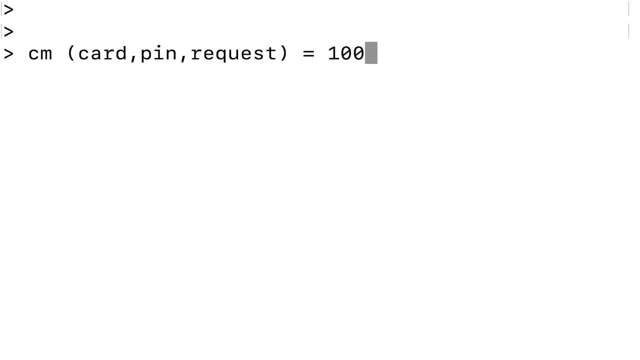 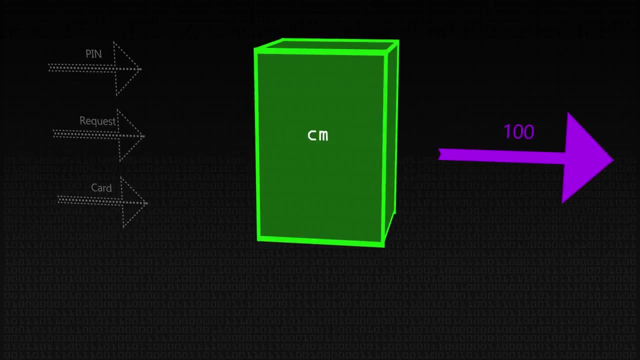 response, which usually is: taking some money out, And let's make this a generous cash machine, Let's decide that it's always just going to give you 100 pounds or $100 out, But this is not actually how it works. So if you talk to a cash machine, you don't put all of the three inputs in at exactly the